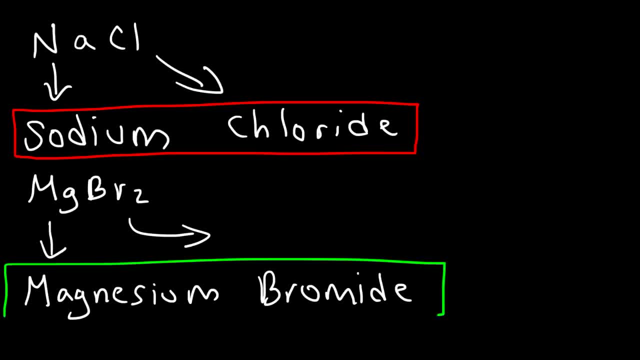 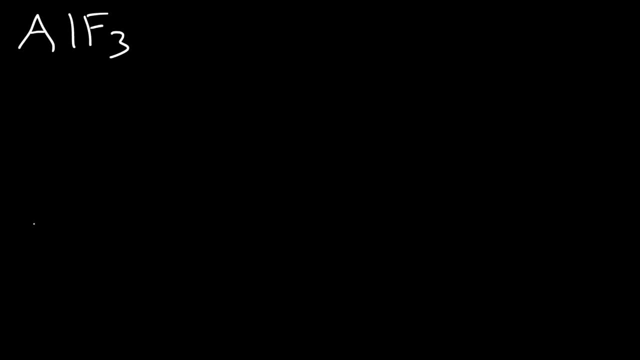 So to name it, it's simply called magnesium bromide. Let's try some more examples: AlF3 and CaO. So Al stands for aluminum, F represents fluorine, But we're going to say fluoride, So AlF3 is called aluminum fluoride. 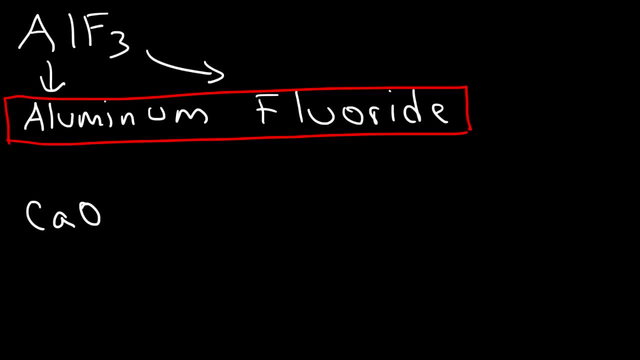 Now what about CaO? What is the name for that? Ca stands for calcium And the O represents oxygen, But we're going to say oxide, So this is called calcium oxide. Now let's try two more examples. Write the chemical names of Sr3N2 and BaS. 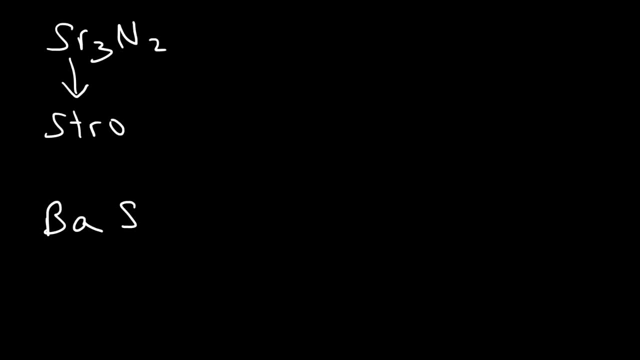 So Sr stands for strontium, N represents nitrogen, So this is going to be called strontium nitride. Now, what about the last one, BaS? Ba is associated with the element barium, S is sulfur, but we're going to change it to sulfide, So barium sulfide. 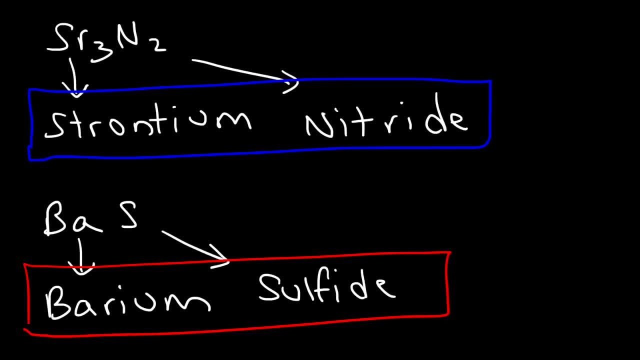 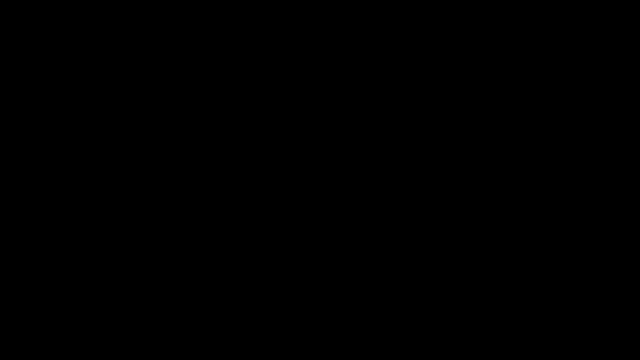 So that's how you can name binary ionic compounds. Now, sometimes you might be given an ionic compound that contains a polyatomic ion, And the periodic table won't help you much in this case, at least for the polyatomic ion. 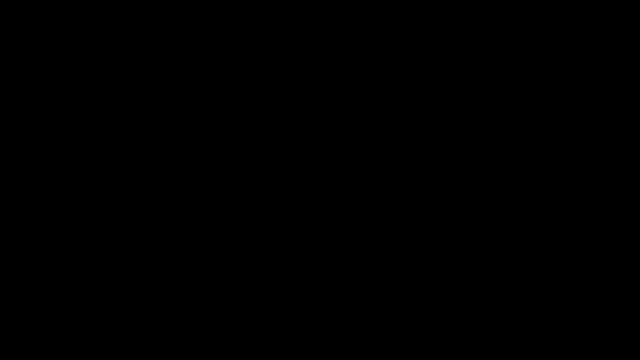 You simply have to commit it to memory. If you're fortunate, your teacher is going to give you the polyatomic ion sheet And so you could just write it down. Just use that, look it up. If not, you have to commit it to memory. 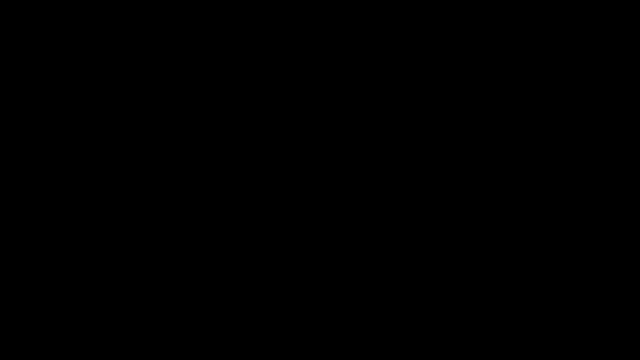 So you're going to need it for the rest of your chemistry course. I would advise you just to memorize it, And it's just going to make life easier. So let's start with Li2SO4 and Na2CO3.. So how can we name this substance? 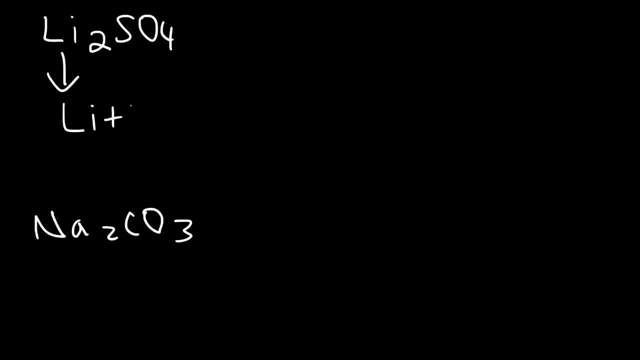 Li, you could look that up in the periodic table. That's a lithium. Now, SO4 is a polyatomic ion. It has a single name. The periodic table won't help you with that. You need to look it up in your polyatomic ion sheet. 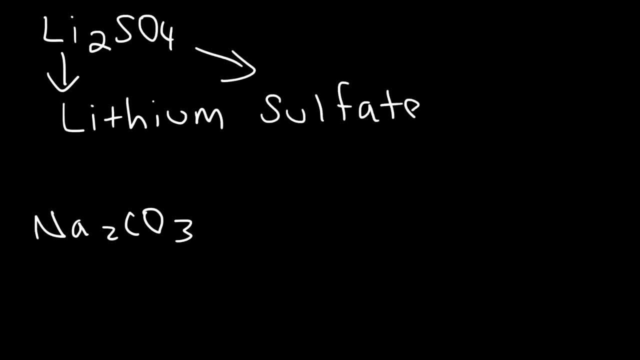 SO4 is simply called sulfate, And that is something you just have to know. Now there's a video in which I made that goes over the common polyatomic ions that you need to look for. Just look it up on YouTube, You should be able to find it. 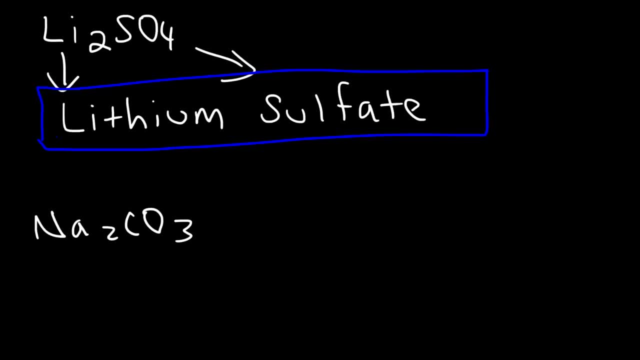 And it's just. it'll help you to understand how to name certain polyatomic ions, So it's easier for you to memorize it. It helps you to get a better understanding of the naming system: Na2CO3.. Na represents sodium. 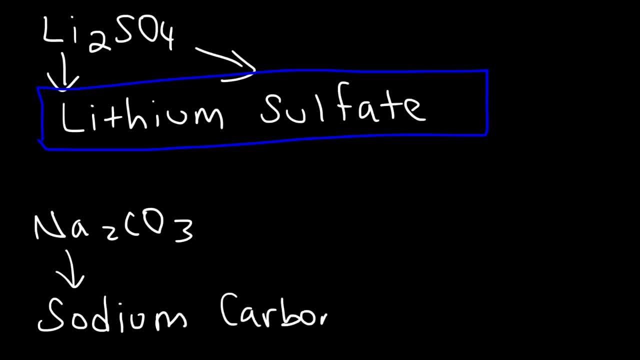 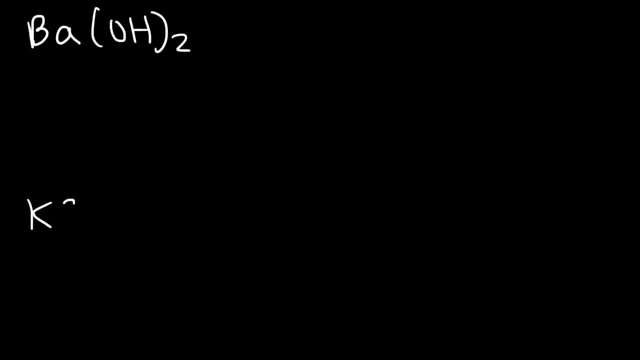 CO3 is called carbonate, So combined it's sodium carbonate. Here's another one Name. this one: BaOH2. And KC2. H3OH2. Or just O2.. Ba is barium And OH. when you see it, it's known as hydroxide. 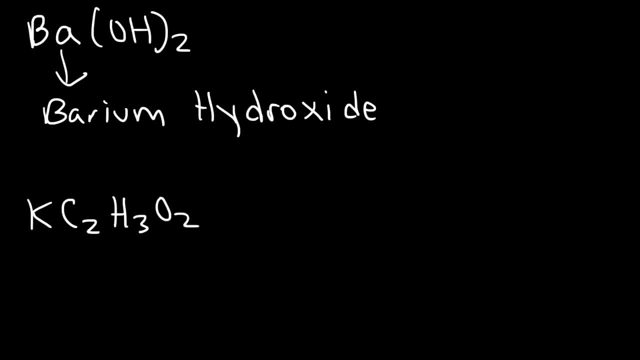 So this is going to be called barium hydroxide. Now what about the next example? What does K stand for? K is called potassium And C2H3O2.. That's a single polyatomic ion known as acetate. 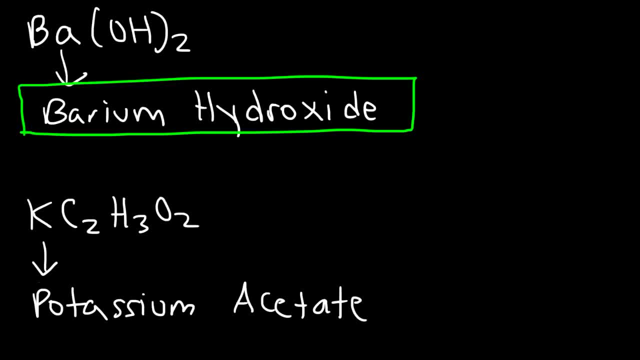 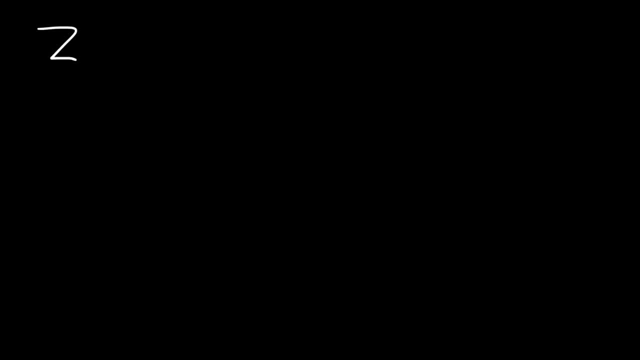 So combined, this is potassium acetate. Now I'm going to give you two more examples with polyatomic ions. Go ahead and name this one, And also NH4NO3.. Zn stands for zinc, ClO4.. NH4 is known as perchlorate. 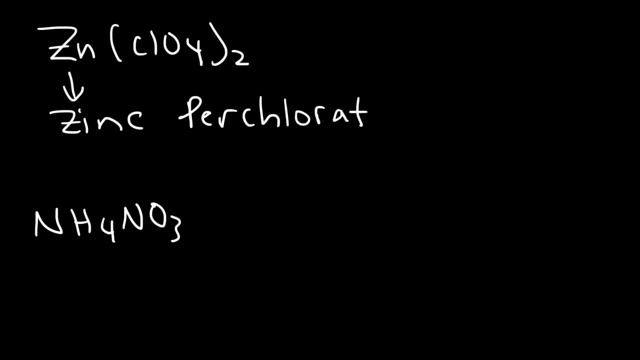 So collectively, this is zinc perchlorate. Now the last one. it's ionic compound, even though it doesn't have a metal inside of it. NH4, that's known as ammonium. That's a polyatomic ion. NO3 is another polyatomic ion, which is called nitrate. 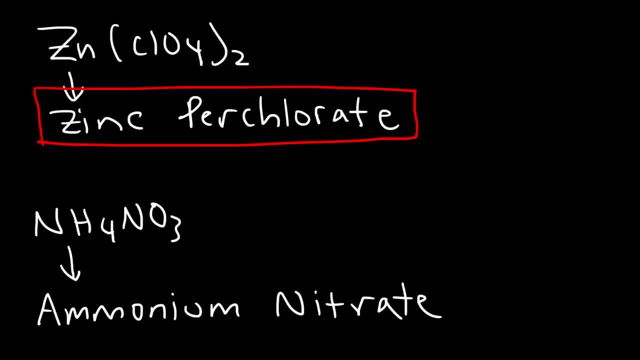 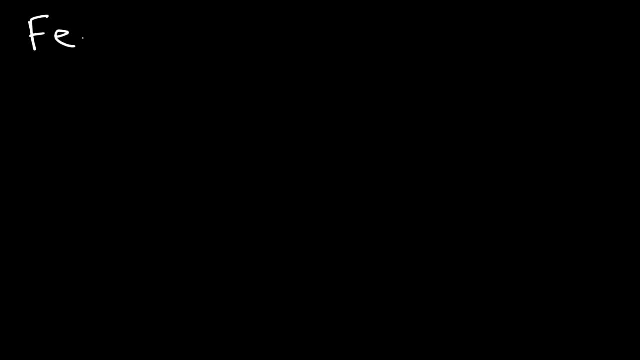 So combined, this is ammonium nitrate And NH4 is zinc perchlorate And NO3 is another polyatomic ion which is zinc perchlorate. Consider these two compounds, FeCl2 and FeCl3.. How can we name these two compounds? 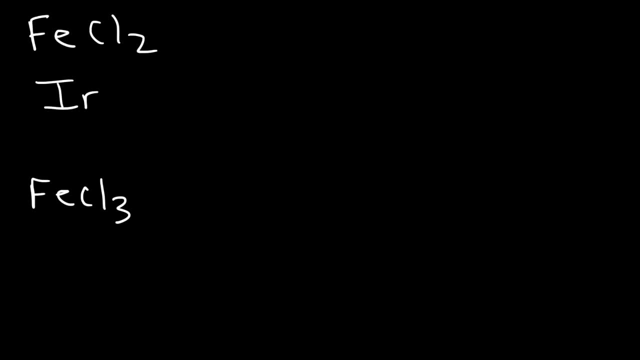 Fe stands for iron, And Cl is going to be chloride instead of chlorine. But now how is this going to be different from the other one? Because the other one is also iron chloride. So we need a way to distinguish FeCl2 from FeCl3. 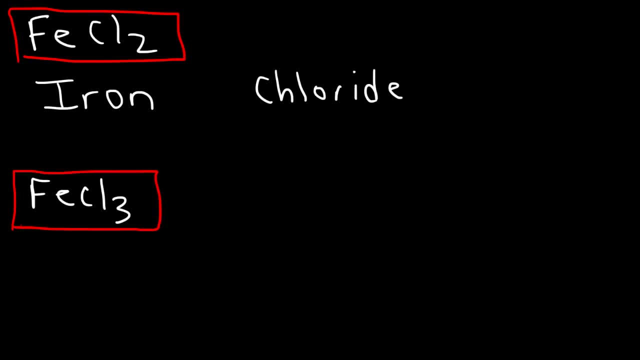 It turns out that certain transition metals have multiple charges, And so you need to use Roman numerals to specify the charge of the transition metal. There are certain metals that are not transition metals that also have multiple charges, And you would still use the Roman numeral system for it. 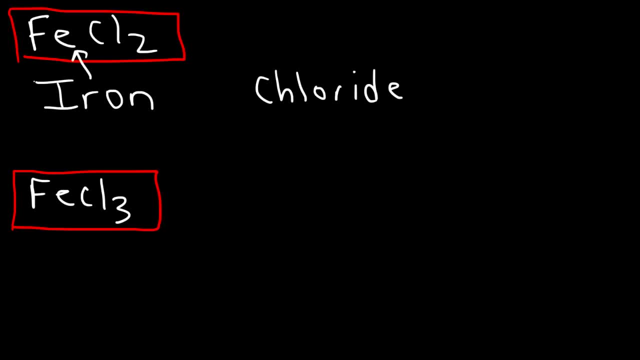 So what we need to do is figure out the charge of Fe and FeCl2.. Now the charge of a single chloride ion is negative 1.. And in this example there are two of them, So the total negative charge is negative 2.. 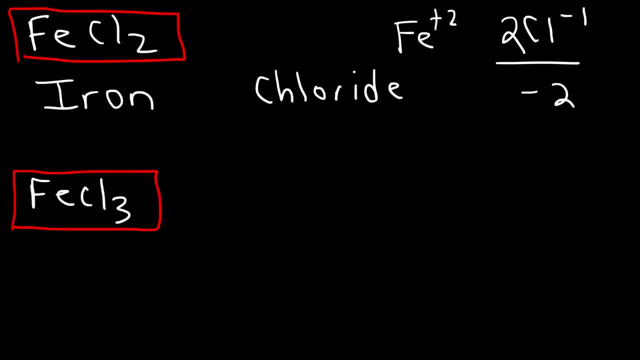 Therefore, Fe has to have a positive 2 charge to neutralize the negative 2 charge from the two chloride ions. So therefore, since there's a positive 2 charge, there's a negative 2 charge from the two chloride ions. Therefore, since the charge on Fe is positive 2, this is called iron chloride. 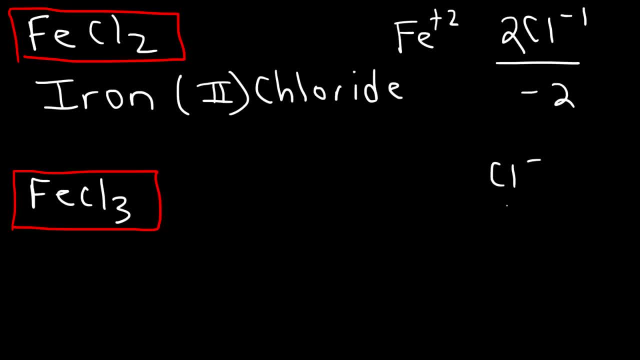 Now in the next example we have three chloride ions. So the total charge is negative 3, which means the total charge on Fe has to be positive 3.. The net charge has to add up to zero because there's no charge on FeCl3.. 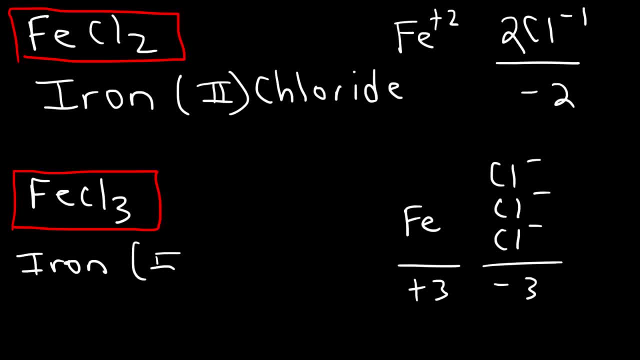 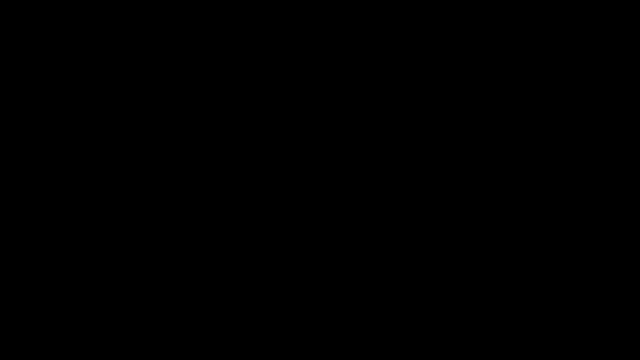 So, therefore, this is going to be called iron chloride, And that's how you can name ionic compounds that have metals with variable charges. Let's look at another example: CuBr and CuBr2.. Go ahead and name these two compounds. 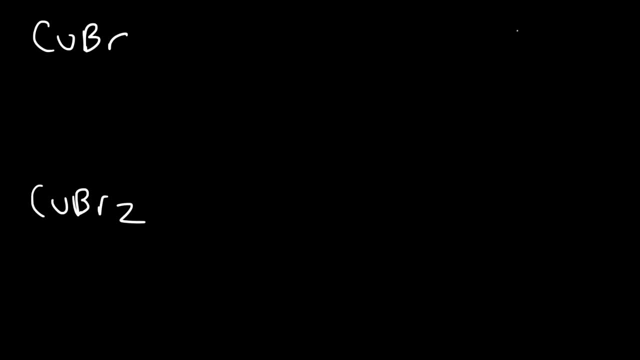 Now let's start with CuBr. Bromide has a negative 1 charge And there's only one of them, So CuBr has to balance that negative 1 charge, So it must have a plus 1 charge. So therefore, this is going to be called CuBr1 Bromide because it has a plus 1 charge. 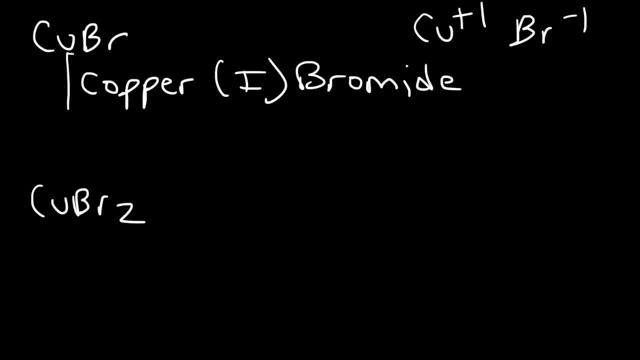 Now what about the second example? What's the name for it? Well, in this case we have two bromide ions, So the total charge is negative 2.. And therefore CuBr has to have a plus 2 charge to balance the two negative charges. 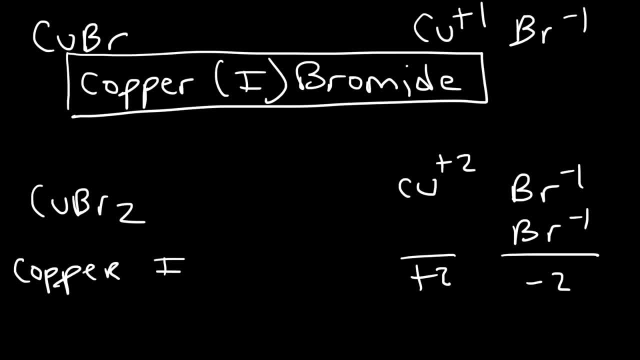 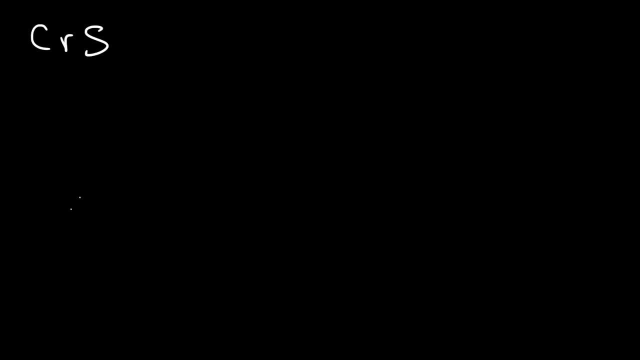 So it's going to be CuBr2 Bromide. Now what about CrS and Cr2S3?? Go ahead and try those two examples. So let's find the charge on sulfur. Sulfur has a negative 2 charge, which means in this example, chromium has to have a plus 2 charge. 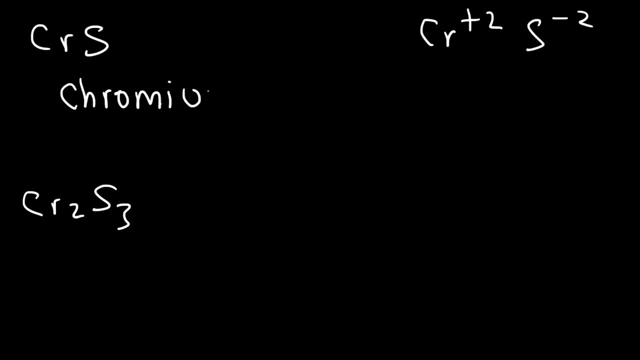 So this is going to be called Cr2S3.. Now for the second example. there's three sulfide ions. So the total negative charge is negative 6.. Which means the total positive charge has to be positive 6.. Now there's two chromium ions. 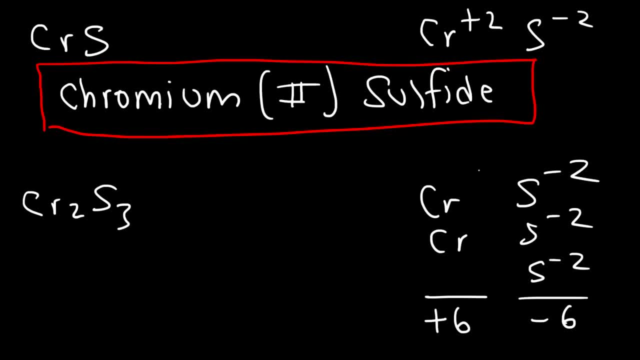 So for the total charge to add up to plus 6,, each of these chromium ions have to have a plus 3 charge. So therefore this is going to be called Cr3S3.. So hopefully these examples are helping you to get this right. 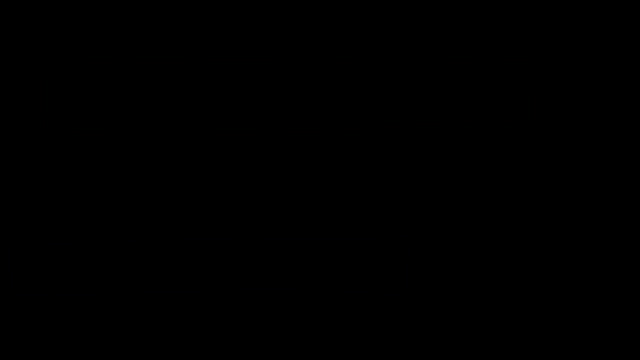 They're helping you. to get a good idea of how to name these types of ionic compounds, Try this: SnO and SnO2.. Oxygen has a minus 2 charge, So tin has to have a plus 2 charge, So the first one is called tin oxide. 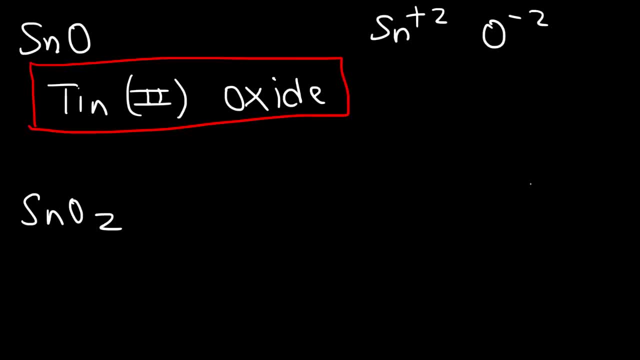 Now let's move on to our next example. So this time there's two oxide ions with a total negative charge of negative 4.. But there's only one tin atom, So therefore it has to have a plus 4 charge.